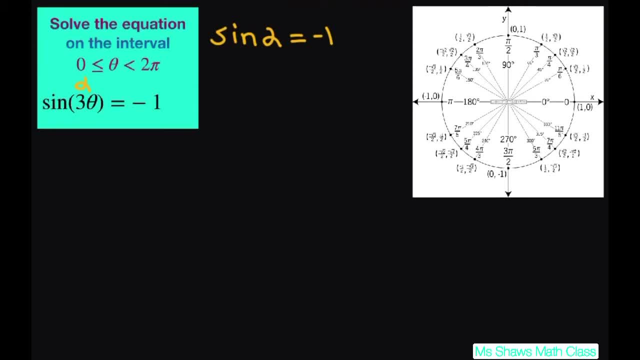 And that's going to be at 3 pi divided by 2.. So our alpha would equal 3 pi divided by 2.. But we don't have alpha. We want this to equal our alpha. So we want 3 theta to equal our alpha. 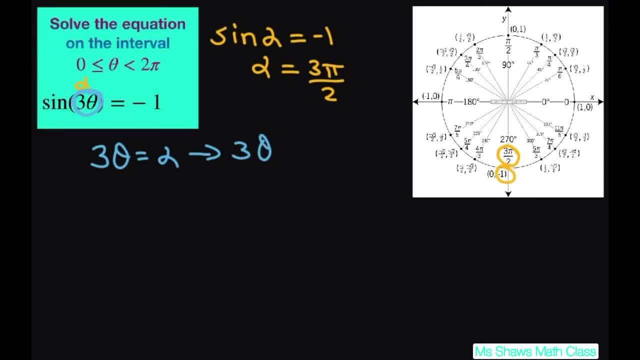 So that means our 3 theta must equal 3 pi divided by 2.. And then we're going to also have to put plus 2k pi, Because we have to get all the solutions on this interval. So now we're going to divide, or let's just multiply everything through by 1 third to solve for your angle. 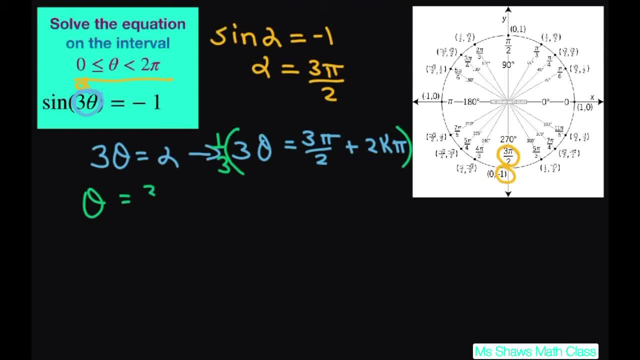 So that's going to give you theta equals 3 pi divided by 6 plus 2k, And that's going to be pi divided 3.. All right, now we have to find all the solutions for this. If I plug in, this would be: theta equals pi divided by 2, plus 2k pi divided by 3.. 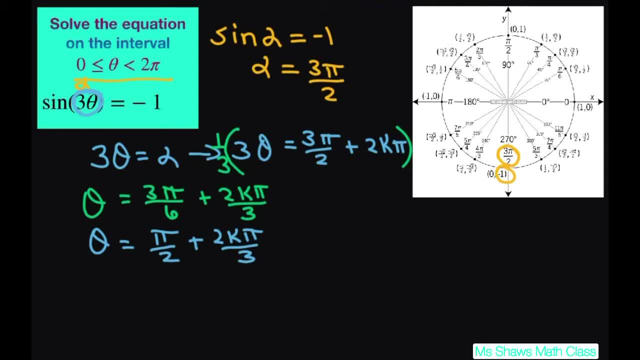 Now let's look and see: If k is 0. I plug in Quiet, plug in 0, this will be 0, so we get theta equals pi divided by 2.. If k is 1, so you plug a 1 in here, you're going to get pi divided by 2 plus 2 pi divided by 3. This 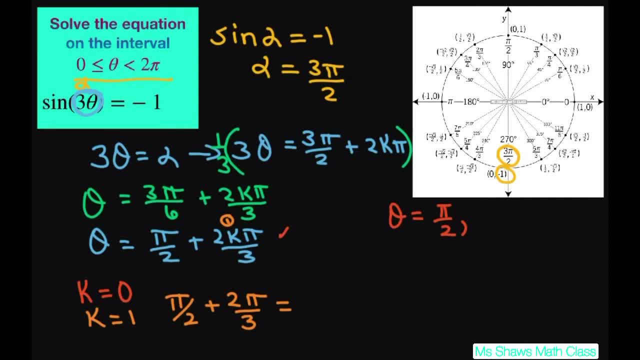 is going to be. common denominator is 6, so that's going to be 3 pi divided by 6, plus 4 pi divided by 6.. That gives you 7 pi divided by 6.. So 7 pi divided by 6.. Alright, let's.